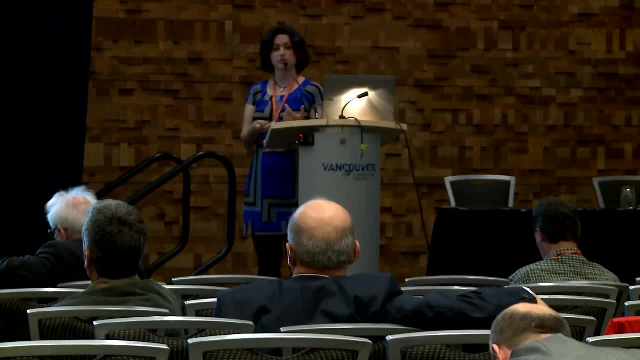 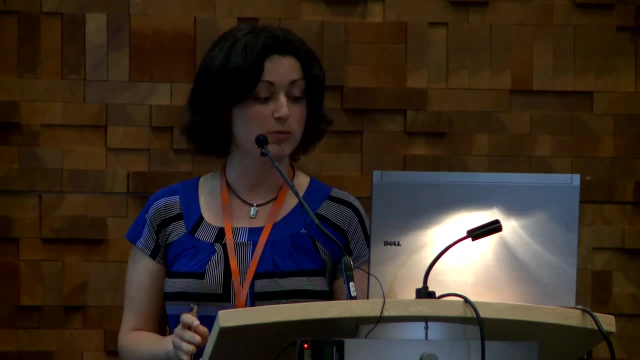 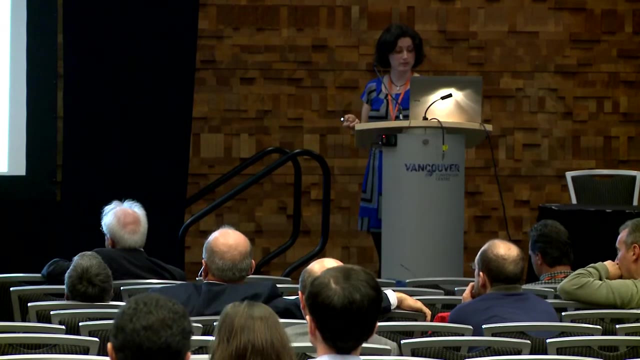 of the process. Cancer is a very complex system, but you can kind of break it down into sub-problems and there you can actually use this very, very well-developed mathematical apparatus to answer targeted biological questions. Therefore, if you know the initial distribution of your clones in the population, then- and 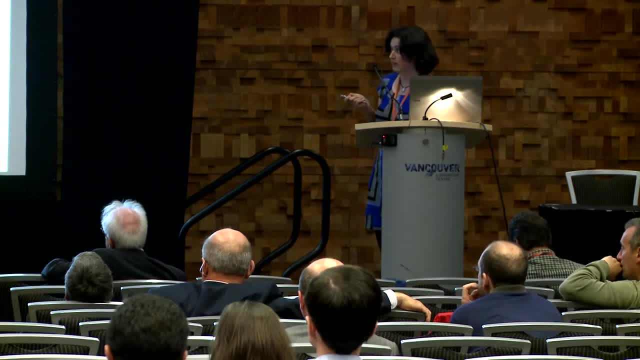 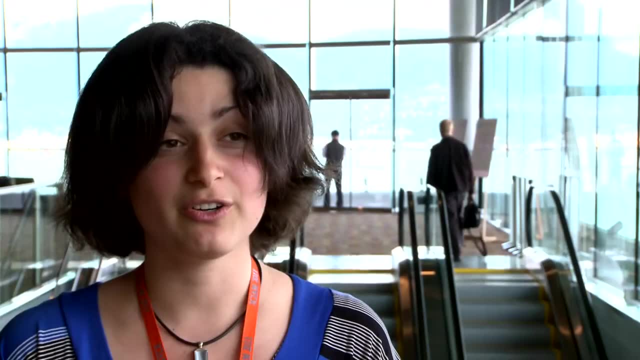 if it has a moment-generating function, Then, using my auxiliary equations that I introduced before, I can calculate the total population size and how it changes over time. In general, what I work on is actually modeling cancer as an evolving ecological system. 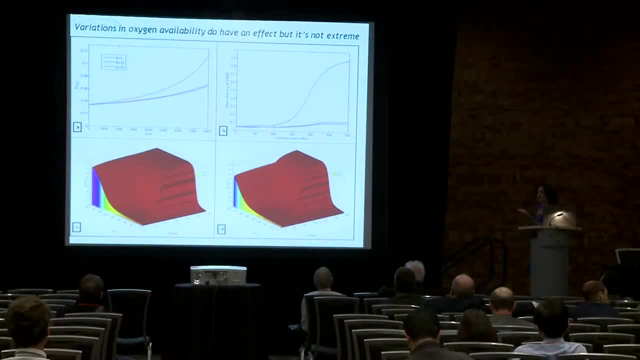 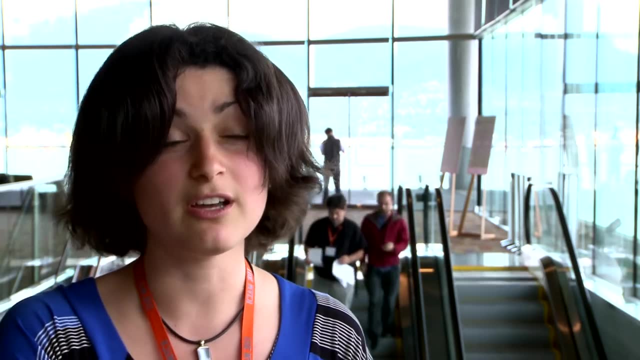 You have a heterogeneous population of cells that compete with each other, with other cells, for space, for nutrients, for all of those things, And we have a very, very well-developed literature on ecology and ecological modeling. What I'm trying to do is reapply that to cancer. 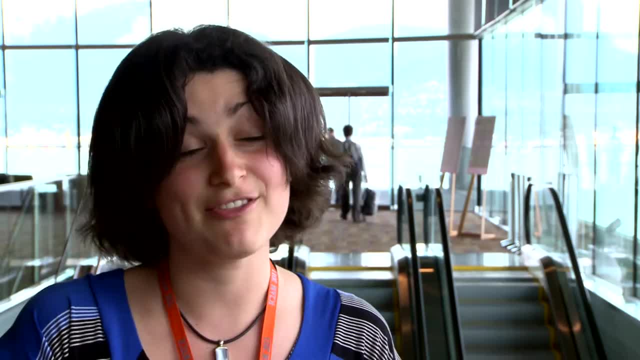 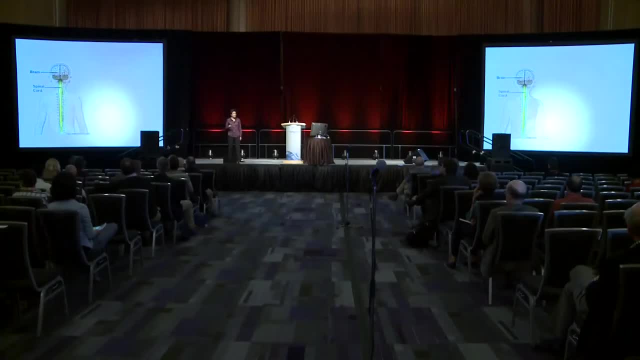 But well, usually we try to save species. In this case we actually want to see. well, what do we know about conservation biology, maybe to try to eradicate this particular subspecies? But we actually have a second brain And this brain unfortunately does not do mathematics. 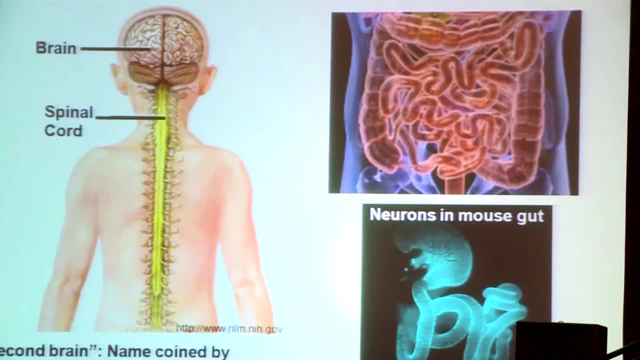 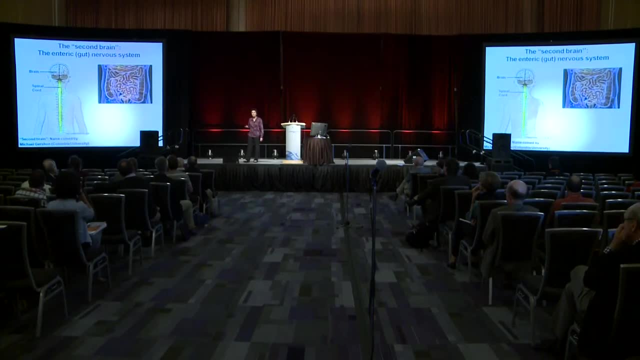 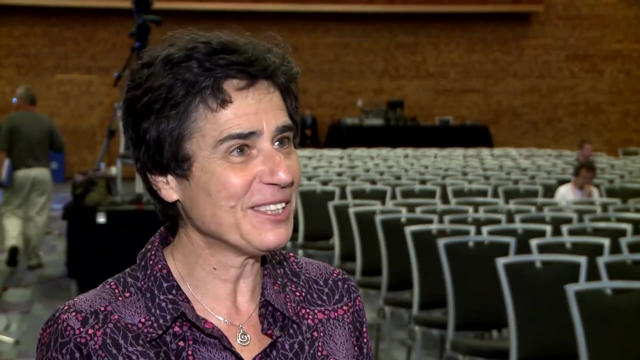 This brain is a large network of neurons which are connected in the gastrointestinal tract and they are responsible for all gut functions. It's a large, complex network of neurons which are all connected together, just like the central nervous system is, And that's why it's called a second brain. 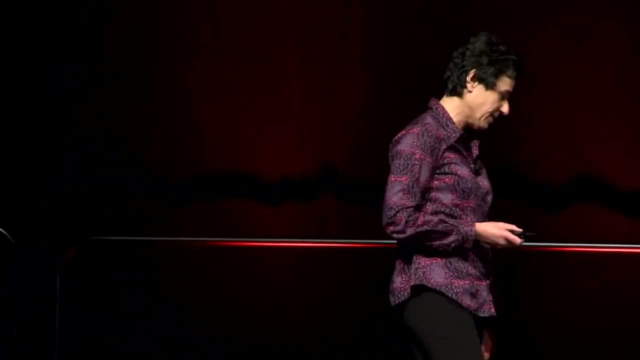 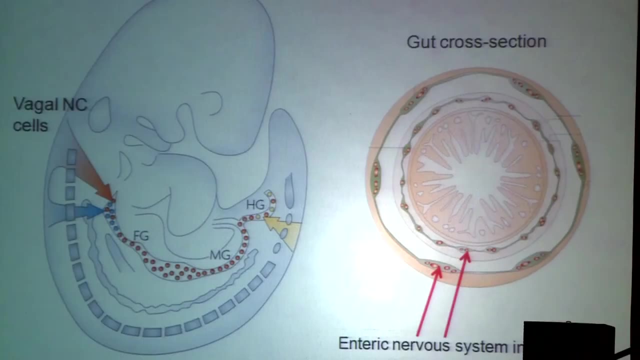 There's a quite common birth defect. it's called Hirschsprung's disease And one in 5,000 babies has Hirschsprung's disease And in this disease there are no neurons in the last part of the gut. 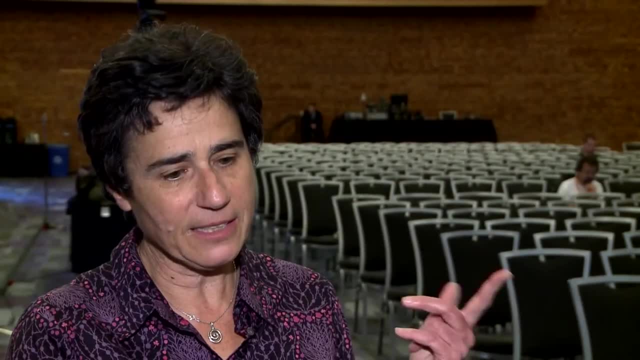 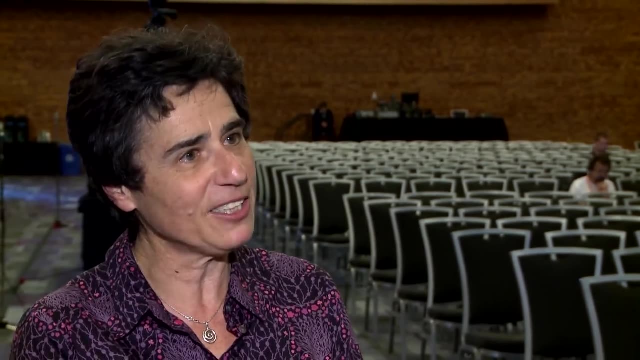 That means there's no peristalsis. This is certainly an example of an invasion process And it's got in tissue engineering you certainly have. proliferation is extremely important and a little bit with migration, And we are working with bioengineers to use some of this in that application. 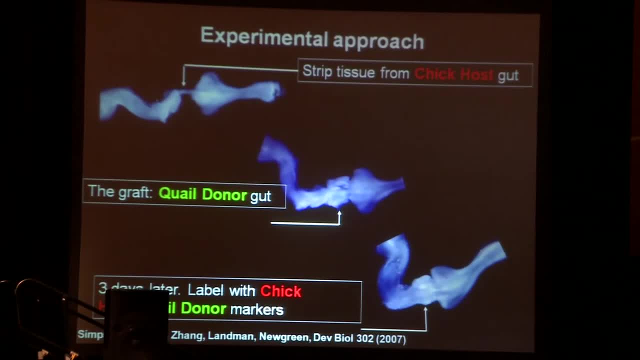 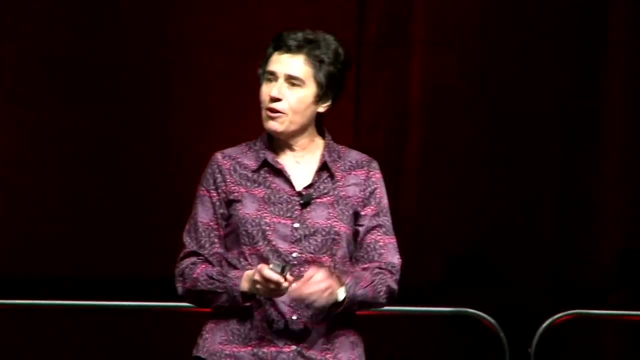 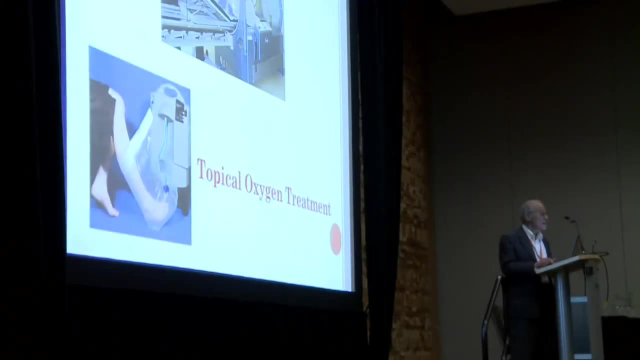 In an experiment, you can't manipulate things so well, whereas in a model, you can play around with parameters and rules that you use, and that allows you to experiment And therefore you can explain experimental data, The primary goal of this particular project.